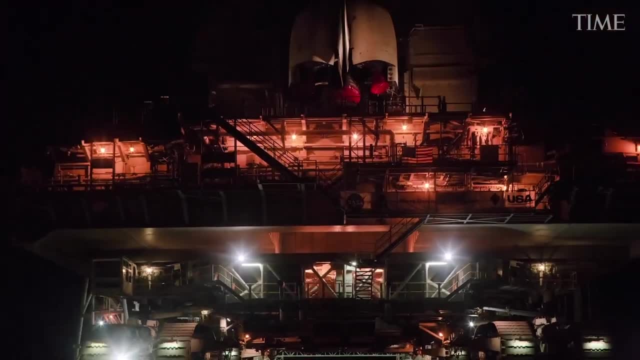 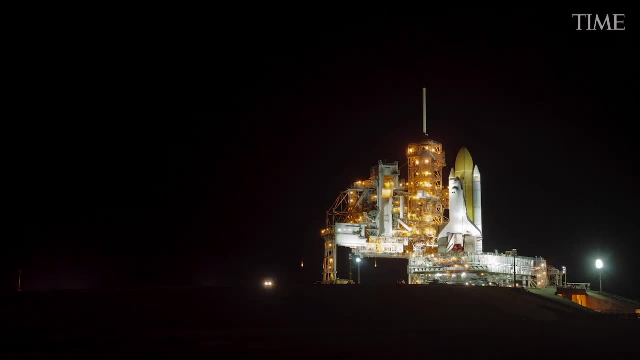 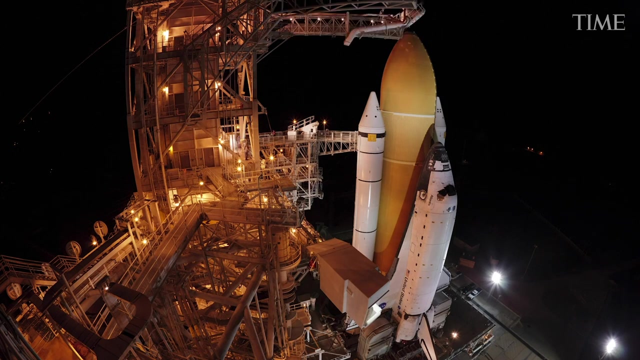 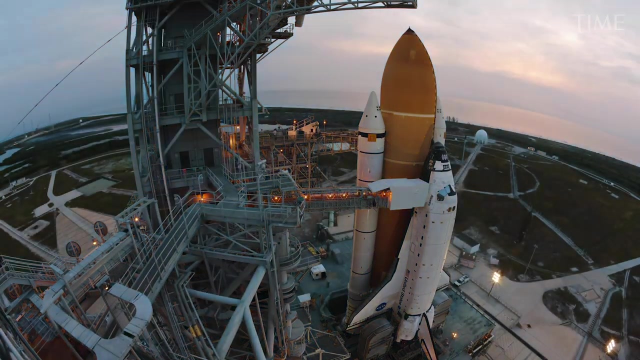 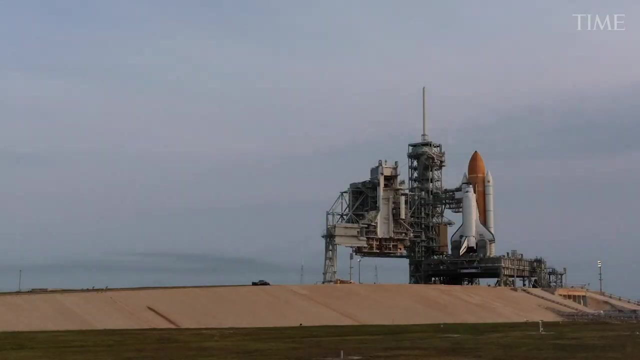 In some ways, its very lack of glamour. It was a reusable workhorse ship that got humans and equipment to and from space and in so doing, helped ensure America's future off the planet. 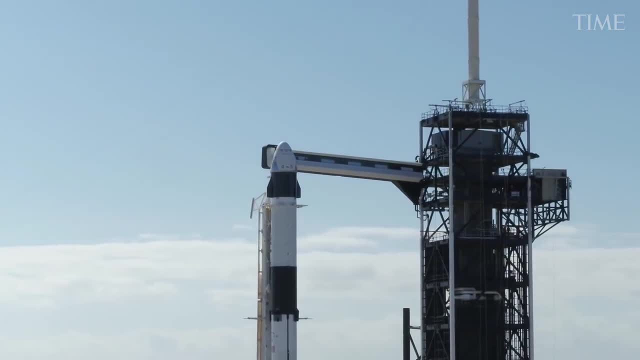 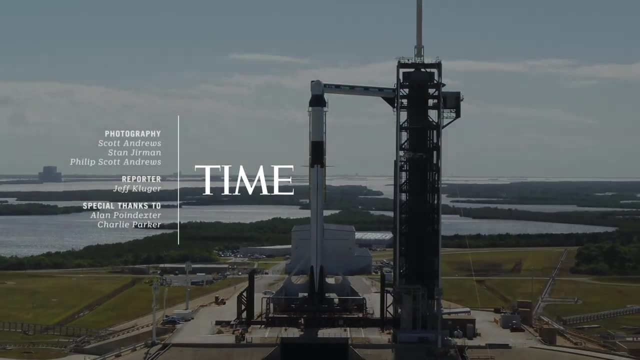 This launch of two astronauts aboard a SpaceX rocket, the first such launch from American soil since Atlantis' flight, is the next big step in that future. Subtitles by the Amaraorg community. 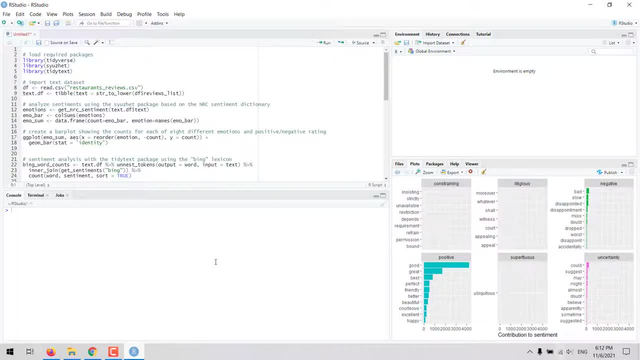 Hello, in this video I'm going to show you how to perform sentiment analysis with the R language. Sentiment analysis is a text mining technique that combines natural language processing and machine learning to assign sentiment scores to the topics, themes or entities within a sentence or phrase. There are a number of packages that can be used for running sentiment analysis in the R. 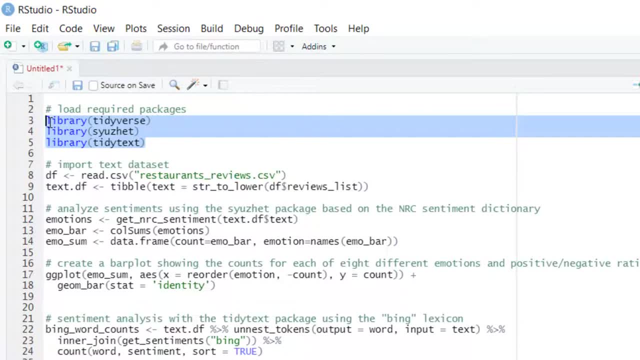 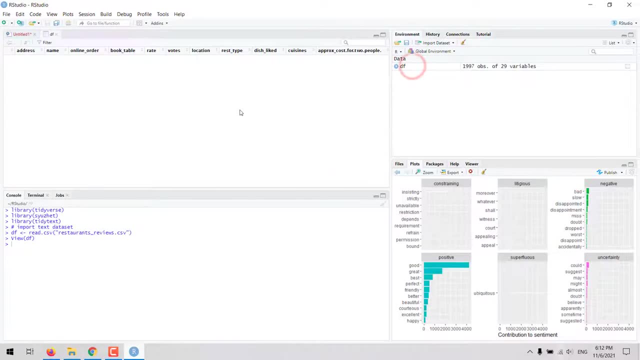 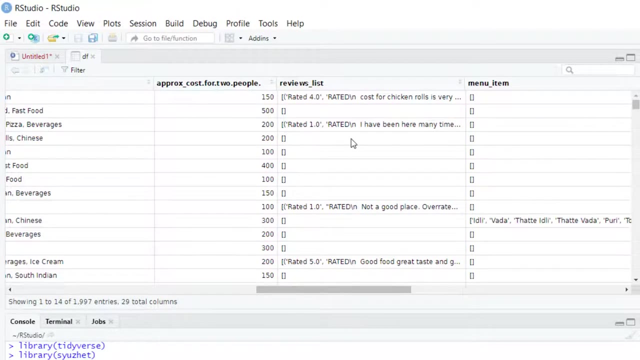 language. I'm going to work with the suzette and tidy text packages For this example. I'm going to use this data that contains information about reviews for a number of restaurants. We have the data for the restaurants and then in this column, reviews, underscore list, we have one or more reviews. 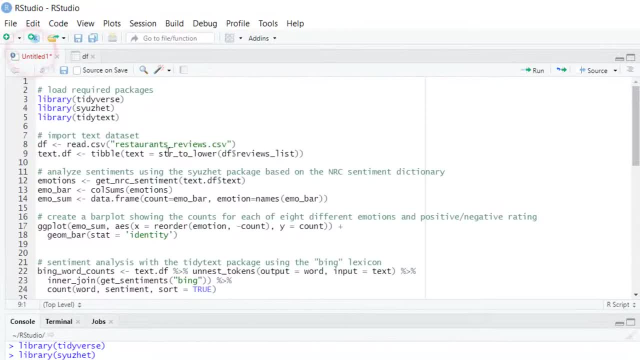 for some of these restaurants. As a first step, I'm going to take that column, convert the text to lowercase and make it a table. Let's see an example with the suzette package first. This package is a text mining technique that combines natural language processing and machine learning. 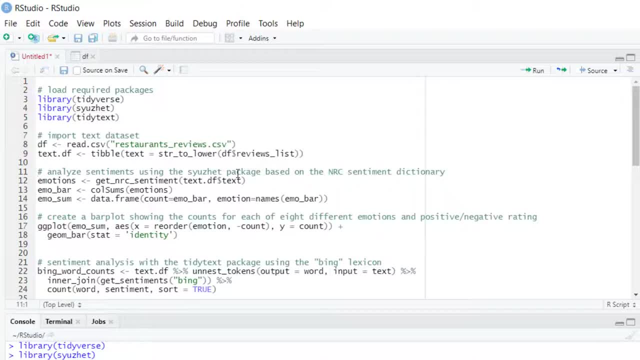 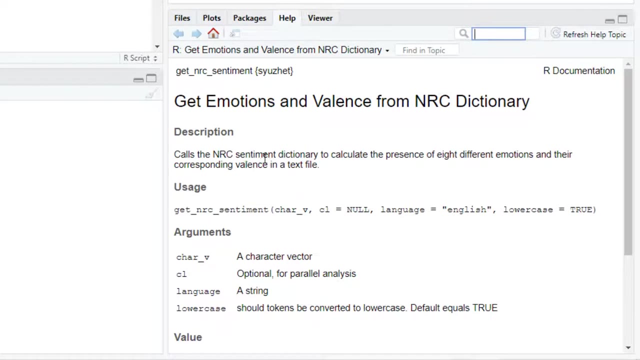 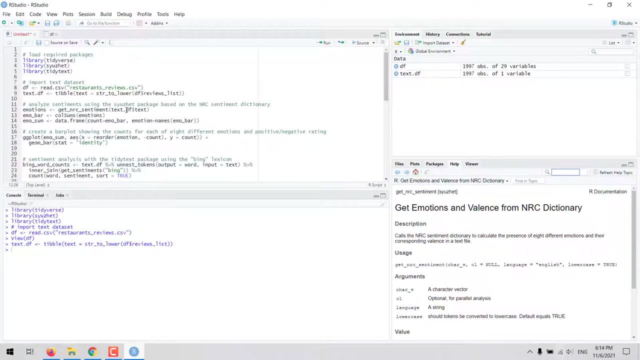 using the nrc emotion lexicon, which is a list of English words and their association with eight basic emotions and two sentiments. The main function here is get underscore nrc, underscore sentiment, which calls this nrc lexicon and calculates the presence of those different emotions and their corresponding balance in a text data set. Let's run that line of code.